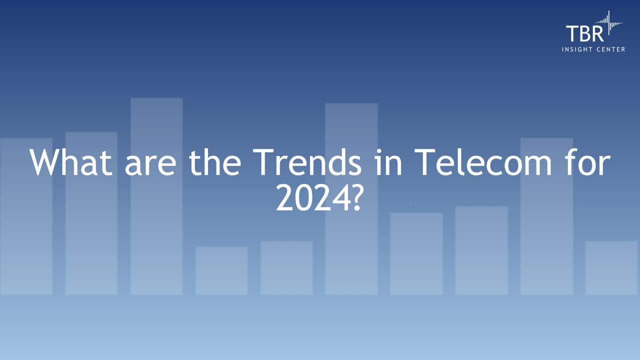 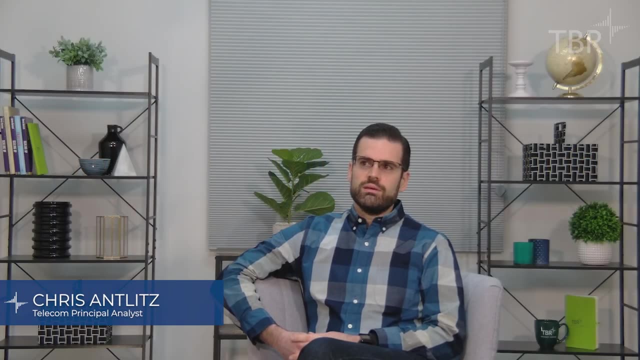 So there's the technology things that are going on in the industry and then there's the non-technology things going on in the industry. So on the technology side we see AI. I think everybody sees AI as top of mind. Also, private networks is a big deal. A lot of people talking about it. We 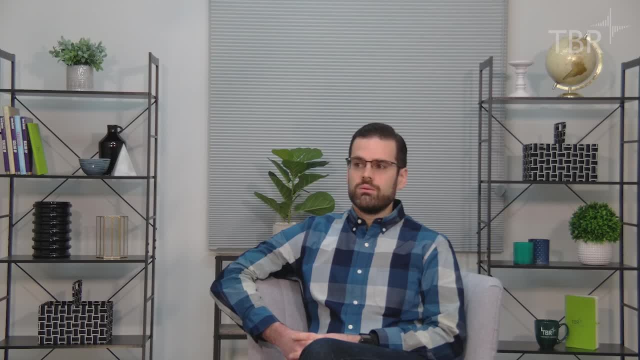 see companies spending money investing in it. We're looking at new disruptive technologies, so quantum computing, how that might impact telecom. We're looking at spatial computing, so how AR and VR is going to change the network industry, Maybe how it's going to be a new 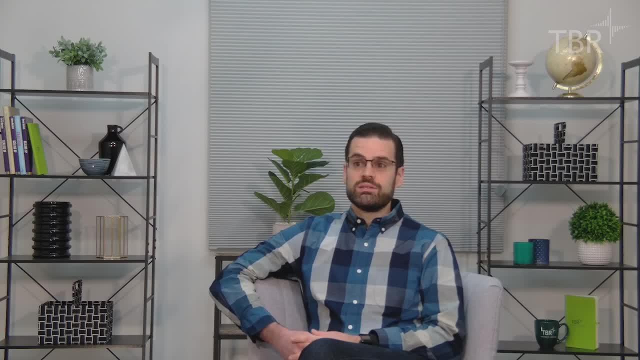 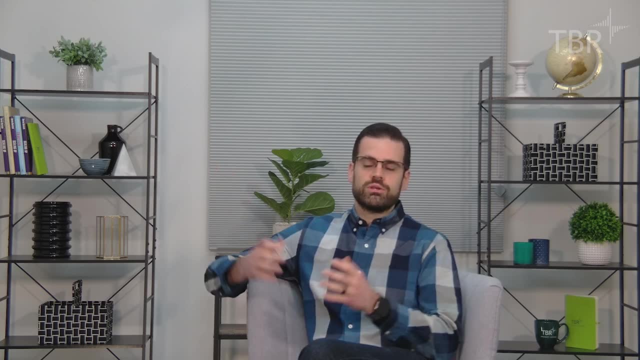 opportunity, but also like the use cases, and how is the industry actually going to support this creation of new technologies? We're looking at how AI is going to be able to support this creation of a quote unquote metaverse. These are some big picture things. 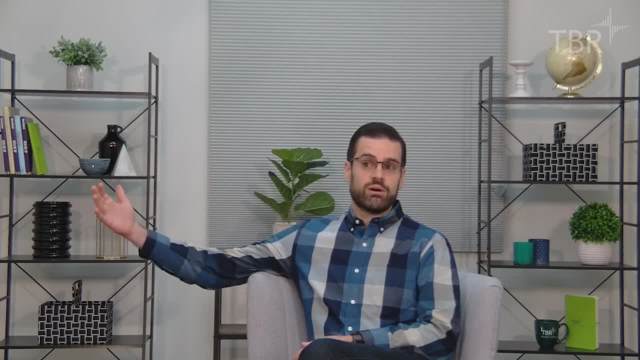 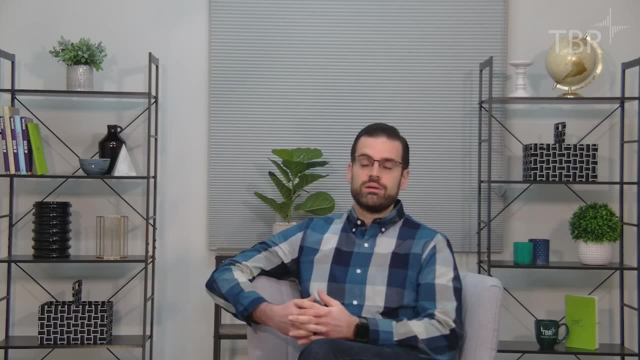 but we are, you know, in our forecasts we look five years out, at least five years out. So we need to be thinking about you know what's coming, and looking at making sure we're keeping pace with that. So that's on the technology side. On the non-technology, 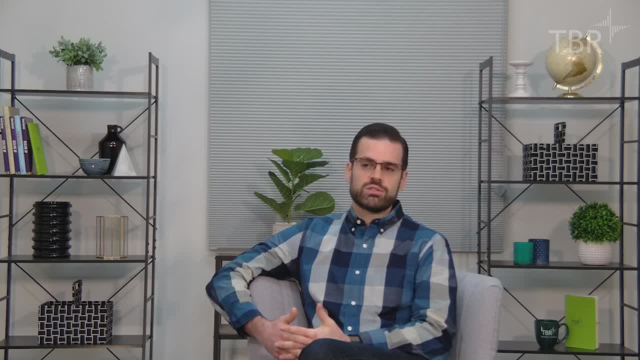 side. it's really about running the business. So we all know the cost of capital is going up. Interest rates have increased quite significantly, especially in the last 12 to 18 months, And, given the high rates of leverage endemic to the telecom industry, this is an issue. 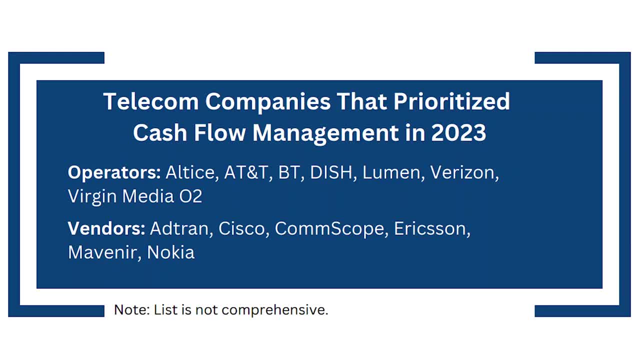 And how are these companies going to manage cashflow? How are they going to manage capex? We are already seeing behavioral changes among telcos and some of the vendors. We are- this is actually one of the predictions for our 2024 document- is: how is the financial? 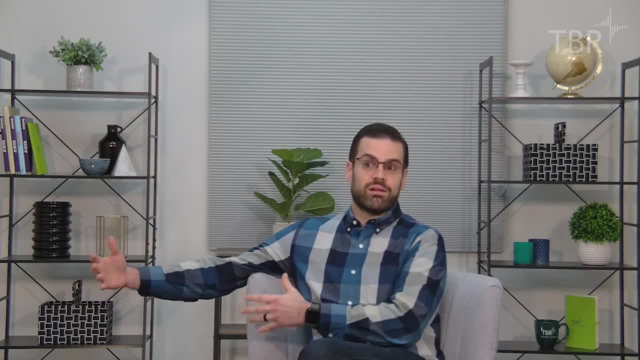 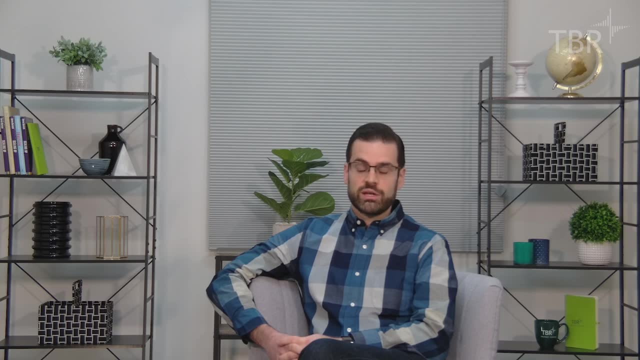 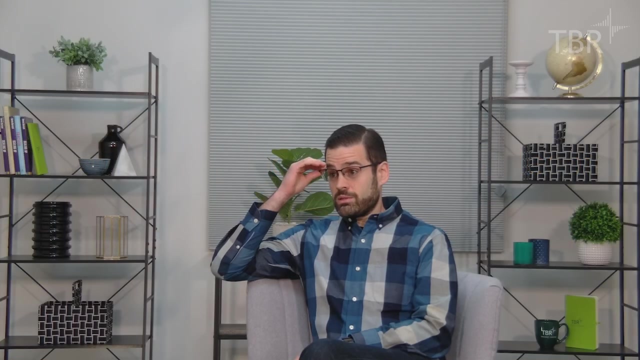 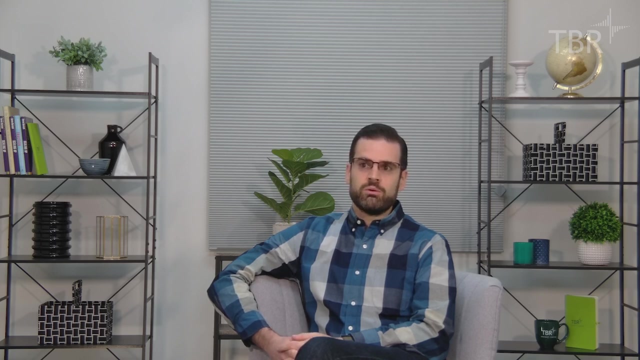 situation, the macro situation going to impact the telecom industry, So that's something we are very much aware of: watching, actively researching. So I've been at this company for 16 years and I am the most excited, coming into 2024, about the